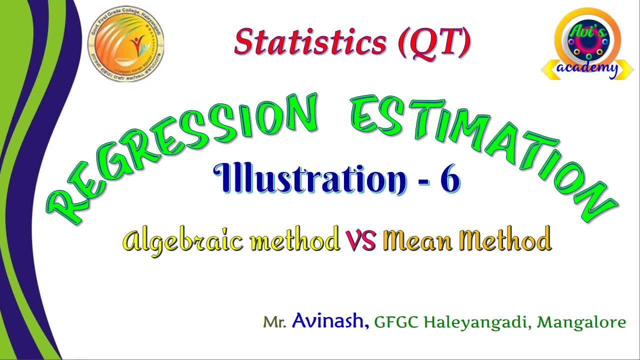 of view saves your time as well, because under algebraic method you have to set few values & then you have to fit normal equations, Then you have to solve the normal equations, then you have positive β & plusで observe, geben H & haben H. 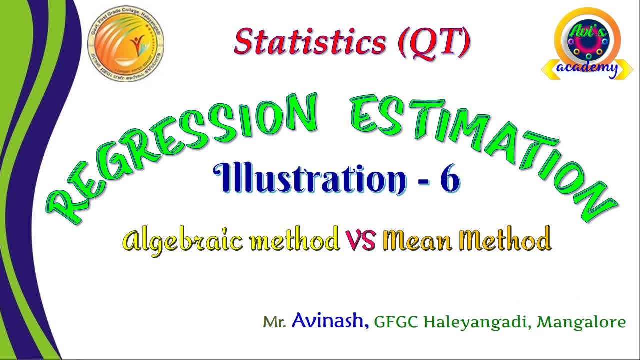 Then rewrite the equation b, 3d, b for al argument of wyst, for includingούμε v2 & för functions with Strategies for scheme & omitted by Ahnungetes a and b value, that is, intercept term and beta coefficient, nothing but the slope coefficient. 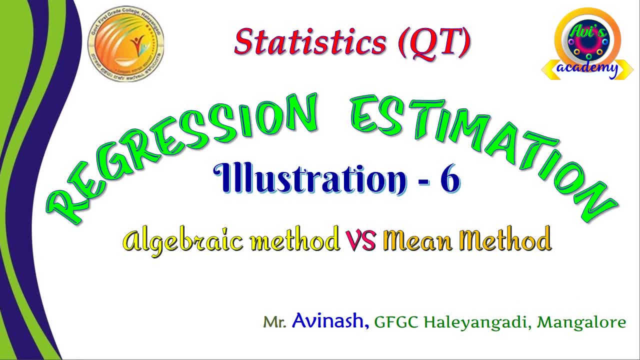 values, whereas in case of mean method we find out certain values. after that we directly find out the slope coefficient, the b value, then we directly fit the regression equation. so it is more simpler than algebraic method. so what we are doing, we are taking an illustration and then we are comparing algebraic mean method. computational aspects of algebraic mean method. 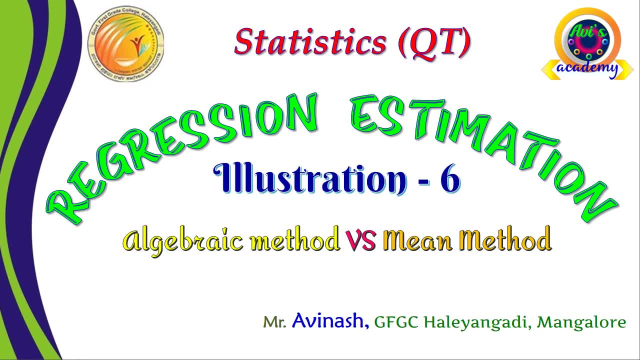 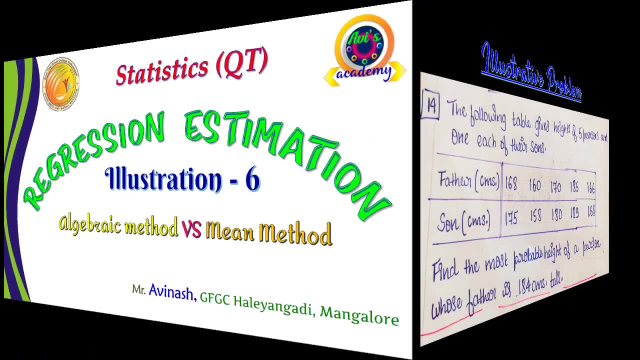 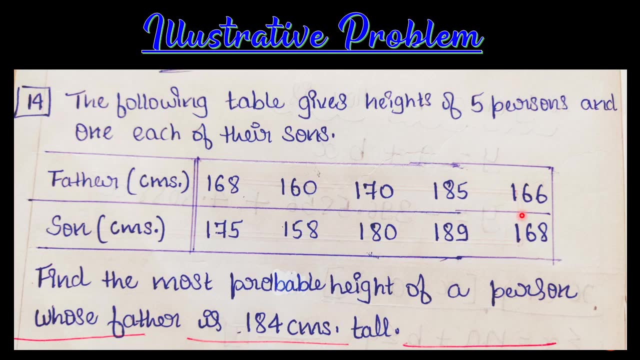 algebraic method and mean method. okay, so let us move on to our next illustration. look at this picture. you have an illustration given. so they said. the following table gives the heights of five persons, and, and, and one each of their sons, which means five persons in height and, correspondingly, our 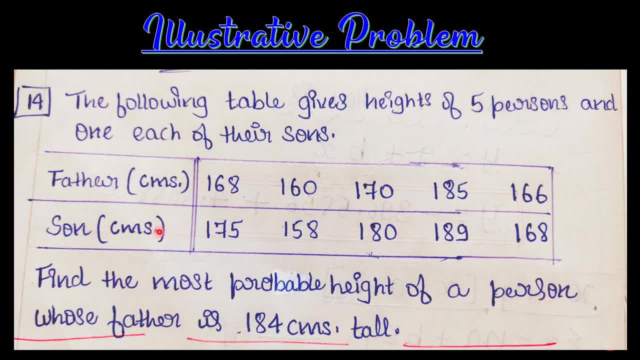 son in height. so you have two values here: father in centimeter. they have given it is actually father's height in centimeter and they have given son's height in centimeter. so values are given. so we have five values of, under each variable, father's height and. 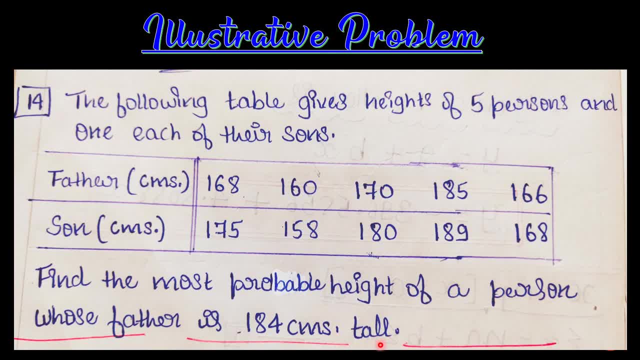 son's height, then actually our question is: find the most probable height of a person whose father is 184 centimeter tall. generally, if you see our previous question, first they ask you to find out the regression equations. then they ask you, then they will give you either x or y values and you arrive at y and x values. 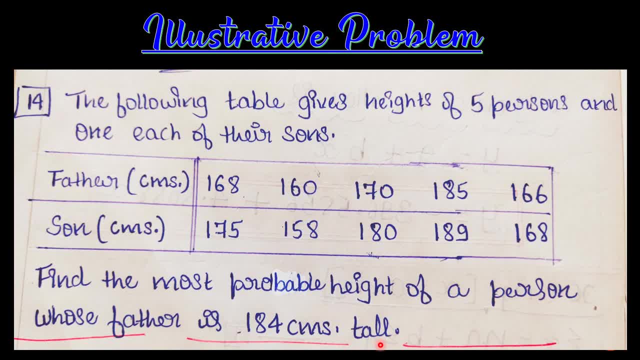 respectively. but here straight away they have given you need to find out the most probable height of a person whose father is 184 centimeter tall. so here they have given the most probable height of a person whose father is 184 centimeter tall. so if you see the variables given father's. 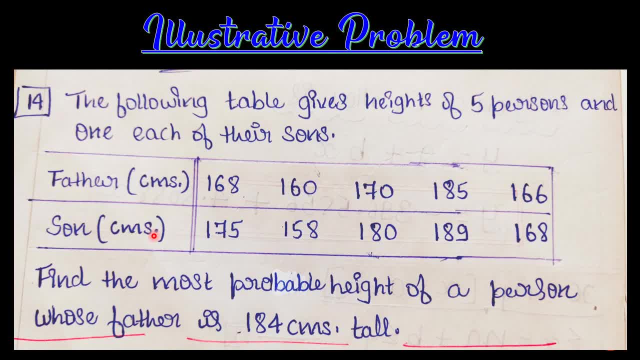 height and son's height. information is available. so i told you, generally when we give information, if any x or y is not clear in the question, if the question is silent about which is x and which is y, what we do generally is we take the first value, whichever is given as 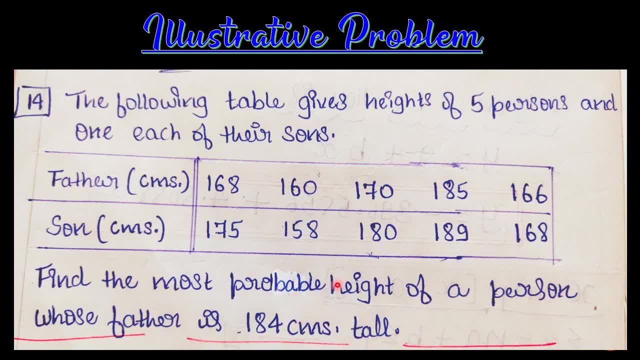 x and the second value as y. if you see the question, they have given father's height. that means we have given father's height. which means we have given father's height, which means we have x value. that it also indicates we need to find out the son's height, which is 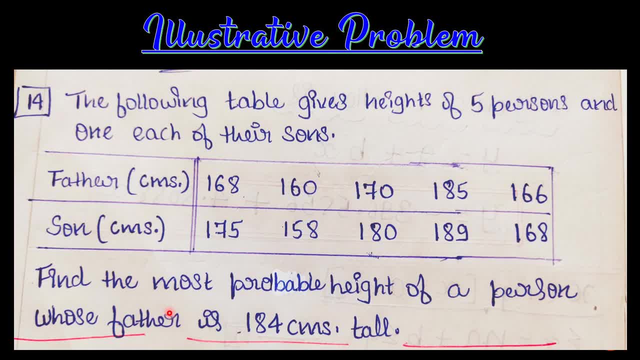 y value. that means we are interested in finding out y on x equation because that will enable us to find out the value for the son's height if the father's height is 184 centimeter. first let's consider algebraic method now. First, the first shall consider the content of the data crossing methodology for the question. 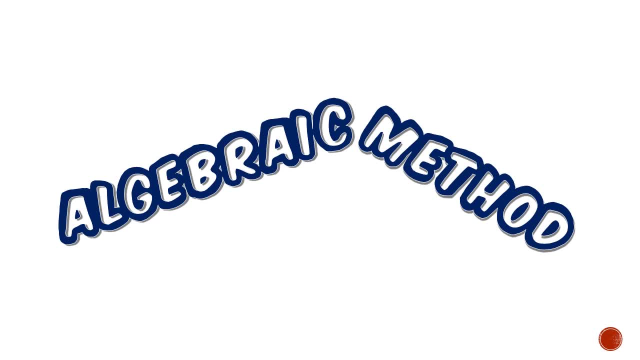 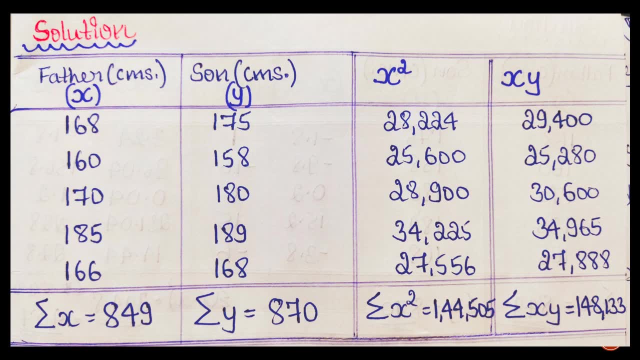 First we will use the algebraic method to fit the regression equation which is y on x. So y on x equation. under algebraic method we need to find out some values. first We have given the information of x and y. After that, to fit the y on x equation, we need x square and xy value. 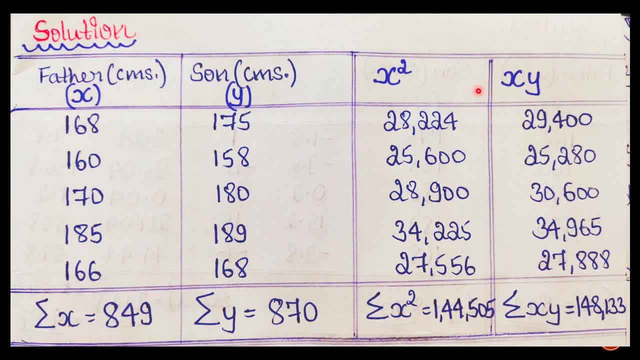 We don't need y square because we don't need to find out x on y equation. So we need these values. So we write x value, then we total it up. We write it as sigma x, which is equal to 849 in this case. 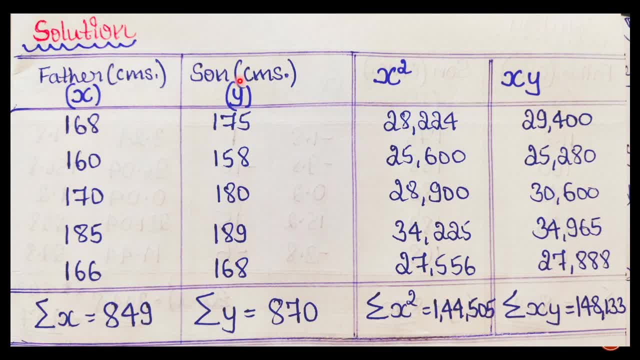 Then we need to find out- we need to write y values, which is given in the equation. Find the sum, represent it as sigma y. After that, we need to find out x square, Because we need to use x square in our normal equation. 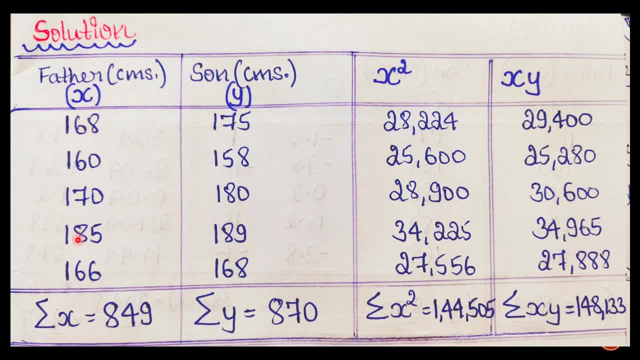 So we have to find this. So we have given x values. We have to square it. So if we square each of the x values, we will get this value. You do that, then find the total, which will be equal to sigma x square. 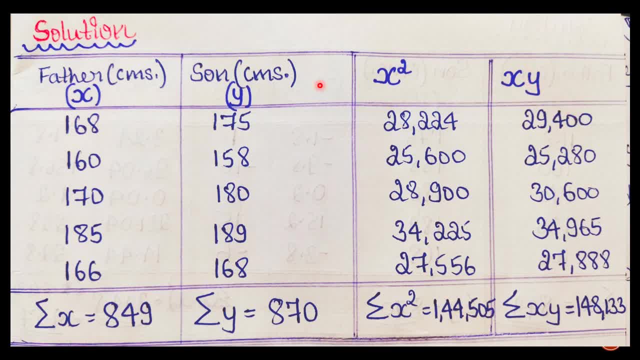 So once that is done, you can find out xy. So x values are given, y values are here. Multiply that. Multiply it, The product. you have to write it here, Then add it up So that will be equal to sigma xy. 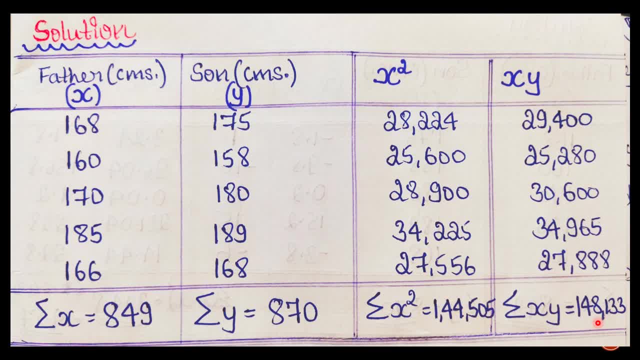 So this is how you need to find out Sigma x, sigma y, sigma x square and sigma xy. So once you find out these values, next we need to substitute each of these values in the normal equation. Okay, So we have to do that next. 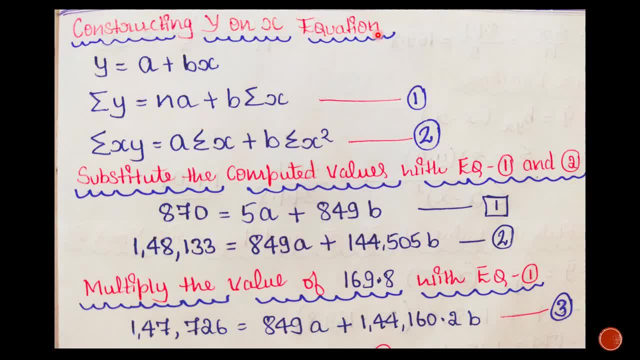 We have to construct y on x equation, So y is equal to a plus bx. Then the normal equation, Because these two normal equations, these two normal equations help us to construct this y on x equation. So we write these two normal equations. 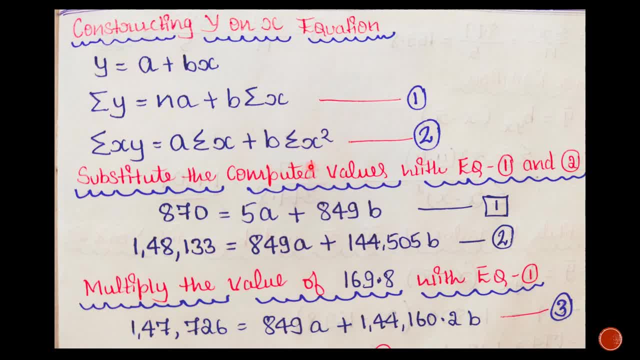 So after that, whatever values we have computed in the tabular format, we have to substitute each of those values with the normal equation. Okay, So we have to find out y, Which is equal to 870.. Which is equal to 5. observations in n. 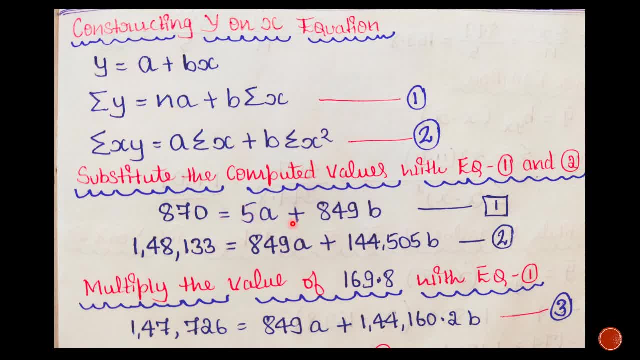 So n is equal to 5.. 5a Plus sigma x: 849.. So 849b. So this is our first equation. Second equation: sigma xy. Again, now find out sigma xy So, which is equal to 148133.. 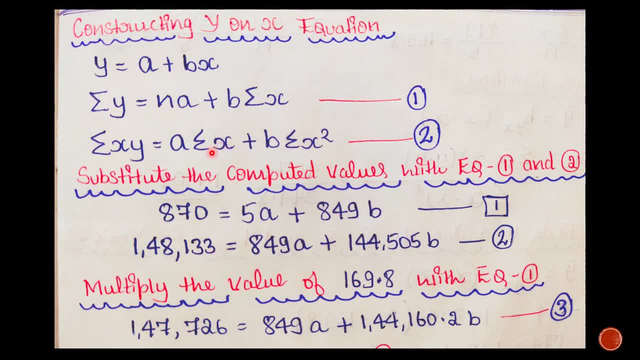 Then sigma xa. into sigma x, Nothing but sigma xa. you can say So 849a. Then you have to find out sigma x, square, also Right, So which is 144505b. So these are our two normal equations after substitution of the values. 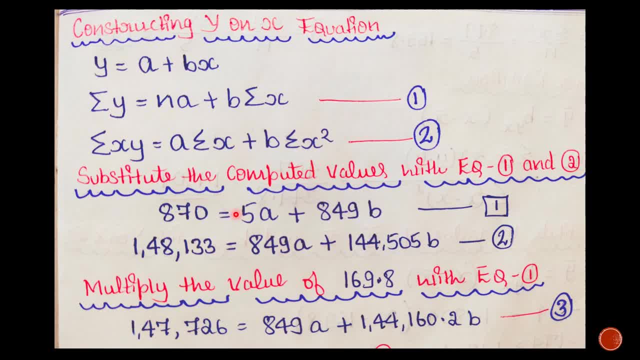 After that, what we have to do next is: here we have different values, Right? We have to make this value same, Right? So what we have to do is we need to multiply a certain factor with this first equation So that the 5a becomes 849.. 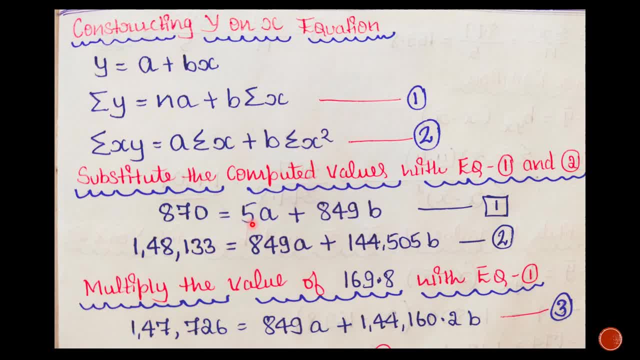 So this becomes 849a. Now again we have to multiply here. Generally, now, arithmetically speaking, we have to multiply from this fractional value. But here we have to take a full value, whole number or integer number, Because here we have to use fractional values, because we do all the calculations. 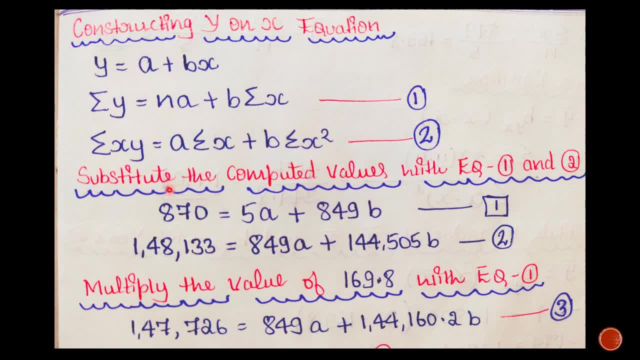 Because we have to multiply this with each of these values Right Now. when we use a calculator, our calculation becomes easy, So there will be no difficulty Right. So now we have to multiply the fractional values, Not an issue? Okay. 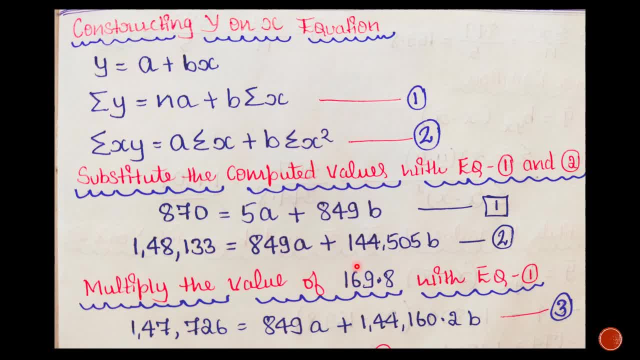 Otherwise they say we need an integer, But this is okay, since we use our calculator in the examination. Okay, So we have to multiply 169.8 with the first equation, So that I have written here: Multiply the value of 169.8 with equation 1.. 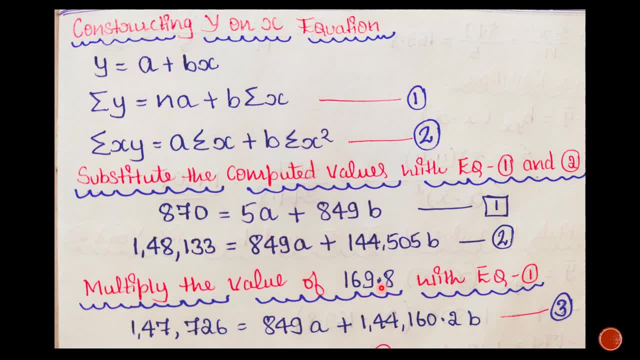 So when you multiply each of the values of the first equation with 169.8,, you get this equation Okay. First, 169.8 into 870. That is how much we get 147,726.. Then multiply these, this value, with 5 and 849.. 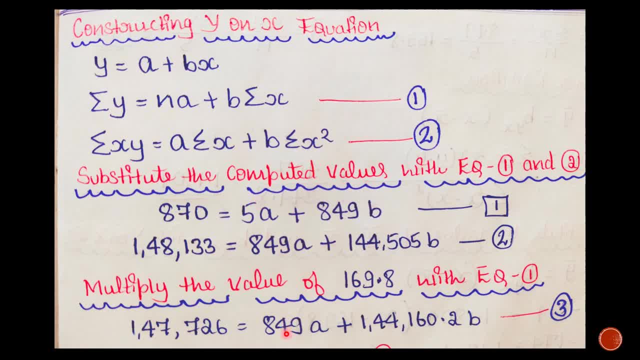 That will result into these two values. Okay, After that, this becomes our third equation. Now, if we check, these two values are the same, So hence we can use it for further computation. We will be doing that now, So next what we have to do: 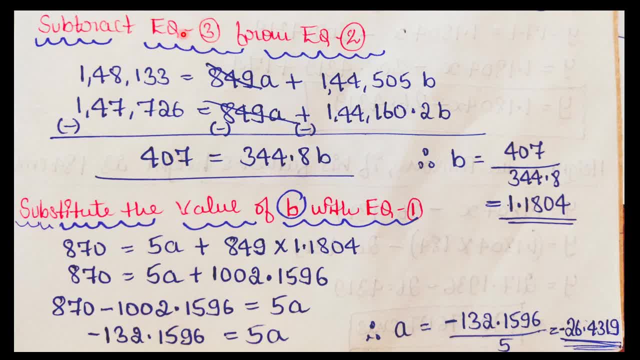 What we have to do is subtract equation 3 from equation 2. So this is equation 2, we have to subtract this from equation 3. So, after subtracting, here is 849 and here is 849, Here is plus 849 and here is minus 849. 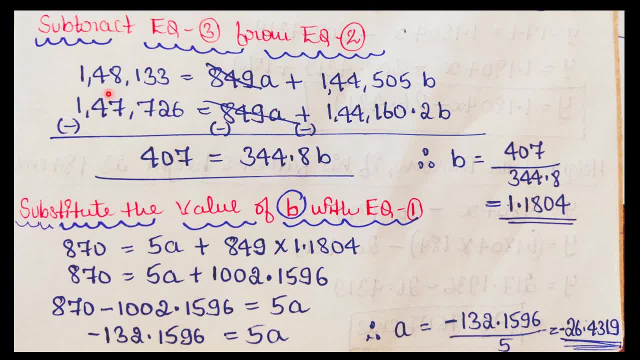 So these two get cancelled. So 1,48,133 minus 1,47,726, which is equal to 407. After that we have to subtract this value from this value, So we get 344.8B. Next we have to find out the value of B. 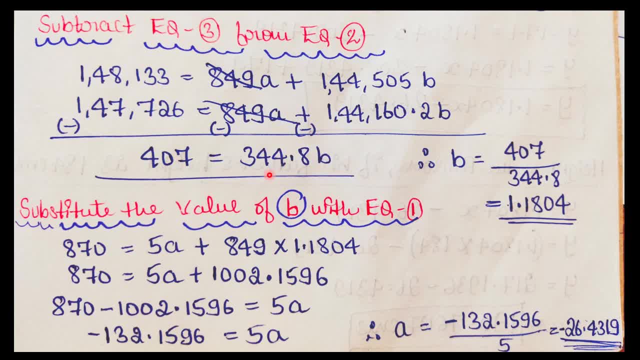 So we have to put B on this side- Here it is 344.8- into B, So when it goes to this side it is 407 divided by 344.8B. So B is equal to 407 divided by 344.8. So therefore B value is 1.1804. 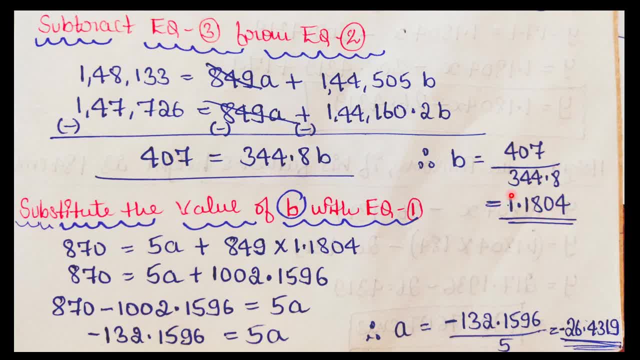 So this is our slope coefficient of y on x equation. So after this we need intercept term, which means A. To find out how to do that, We have to set the three equations of B So we can substitute them. I said previously when I was discussing about algebraic math, 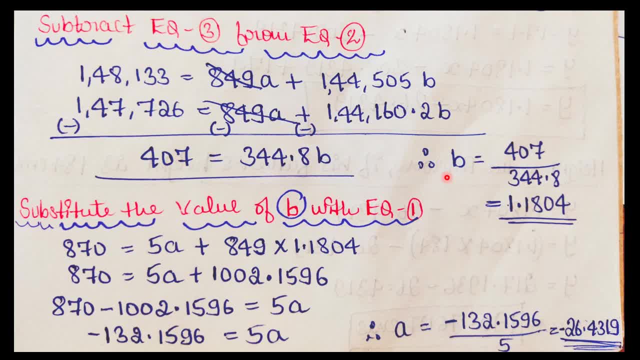 Take an equation where the values are smaller. So generally in the first equation, A First equation will contain smaller values. So we will be substituting the value of B with the first equation. So when we do that we get this: 870 is equal to 5A plus 849B. 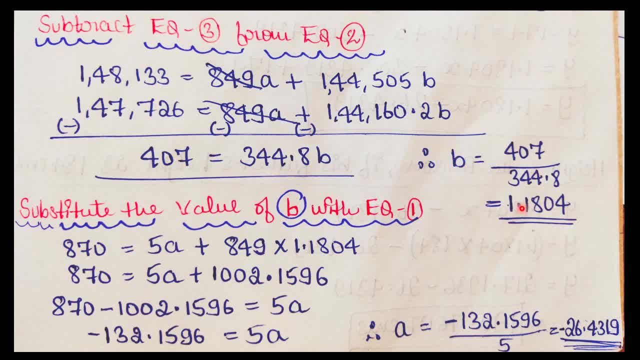 So now I am substituting B's value here, So which is 1.1804. Next 870 remains as it is, Then 5A, Then we are finding the product of these two, Which is equal to 1002.1596. After that, Here we have a different alphabet. 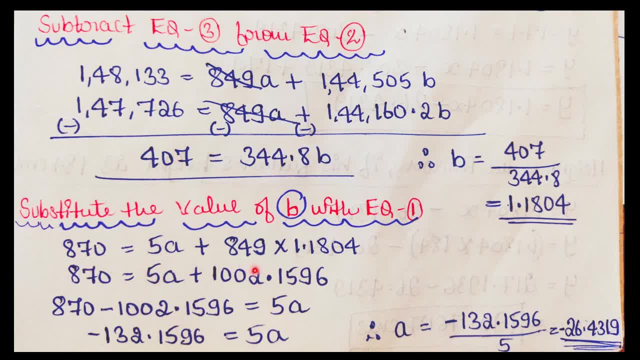 So we cannot add this value to this, Because this is a numerical value. So what we need to do is For the numerical value on the left side. We need to keep it there. So when we do that, Here it is plus. When it goes to the left side, it becomes minus. 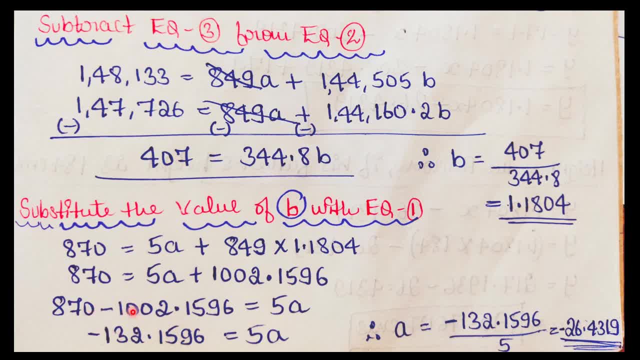 So 870 minus 1002.1596, Which is equal to 5A. So when we subtract here We get a negative value Minus 132.1596. Then we need to find the value of A. A is equal to. When it goes to this side, it becomes divided. 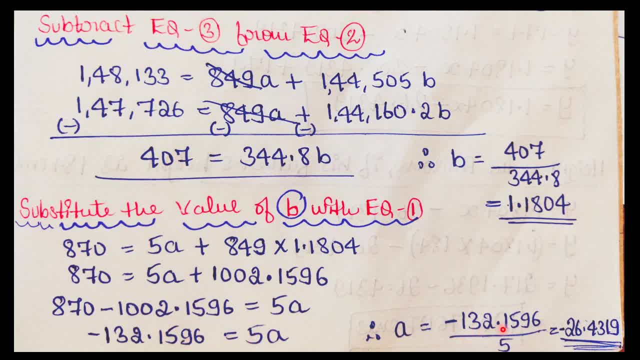 So minus 132.1596 Divided by 5, Which is equal to minus- Remember, don't ignore the sign, Since numerator is minus. Here also it is minus Minus 26.4319. So this is our A value. We got A, We got B. 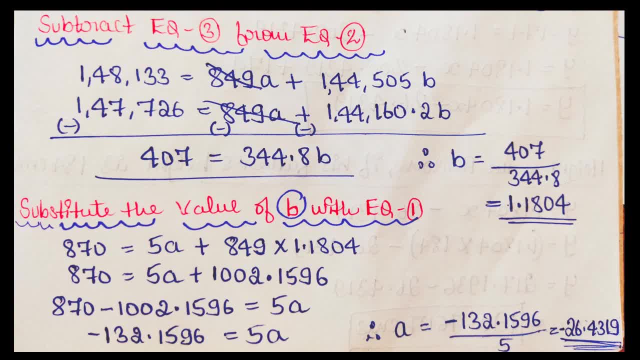 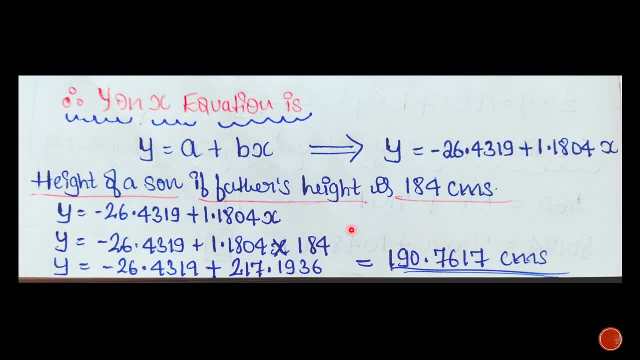 Now directly, you can fit The y on x equation. That we will be doing next. So now fit the y on x equation. Substitute the value of A and B y on x equation. y is equal to a plus bx. So, after substituting, y is equal to minus 26.4319. 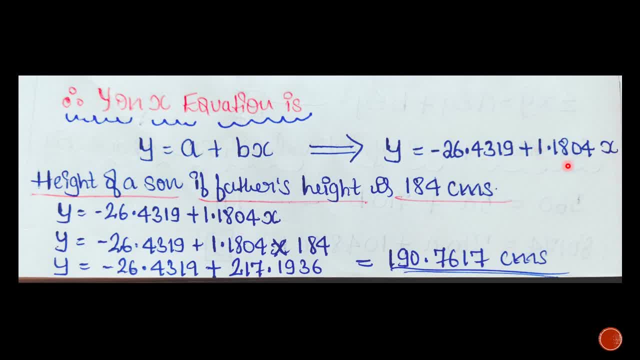 Plus 1.1804x. So next we need the height of a person, That is, son. A father's height is A father's height is 184 cm. So now directly The value of x, Which is 144 cm, When we substitute this in our y on x equation. 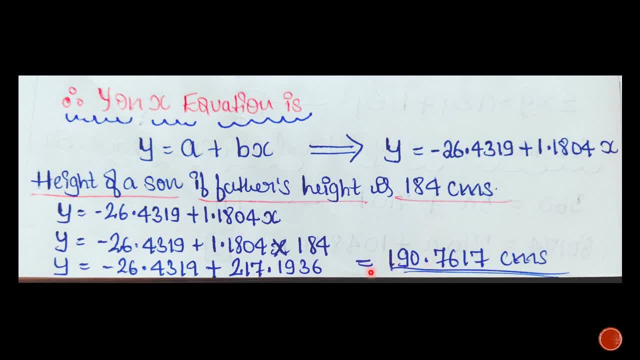 We get the answer. So that will be equal to 190.7617. That means If father's height is 184 cm, As per our regression estimation, Son's height could be 190.7617 cm. This is how we arrive at Regression coefficient Under algebraic method. 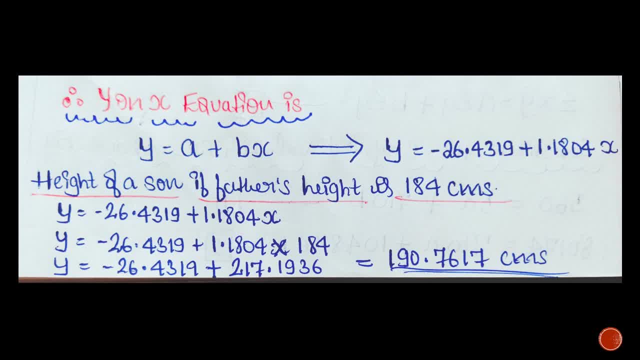 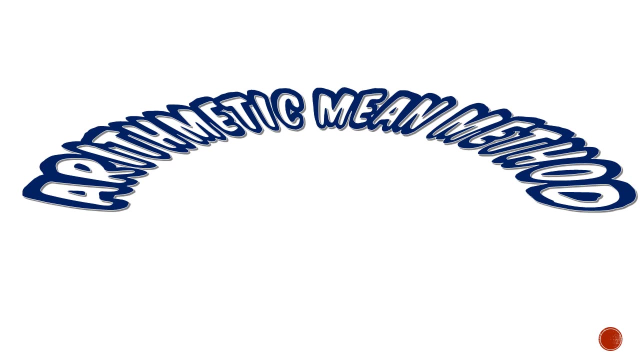 Next, we will take into consideration The arithmetic mean method. We will find out the value under arithmetic mean method. Let us see: will the value be different Or will it be same? Next, we are considering arithmetic mean method. In case of arithmetic mean method as well, We have to find out certain values first. 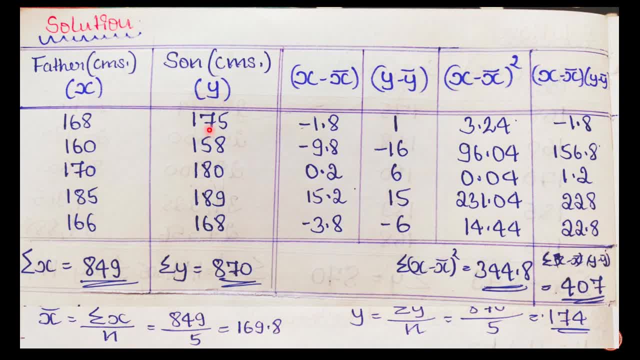 So after this, We have to find out Each of these values To fit that with Regression equation. First, what we have to do is: We have given x values. We will be writing each of those x values. After that We are given y values, So we have to write that. 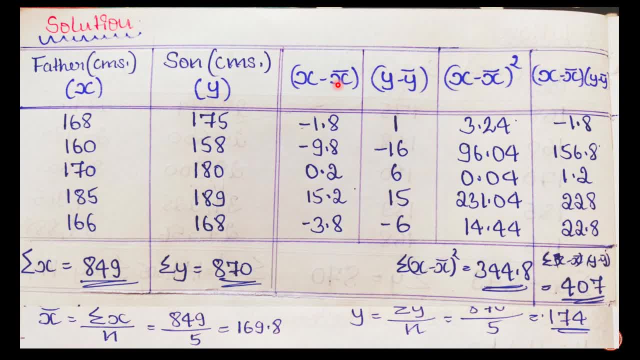 Find the total, Okay, Which is equal to sigma x, As in case of Our algebraic method, Then Find out sigma y. After that, The value we need next is x minus x bar. So we do not know the value of x bar, Which is arithmetic mean. So we have to find that out first. 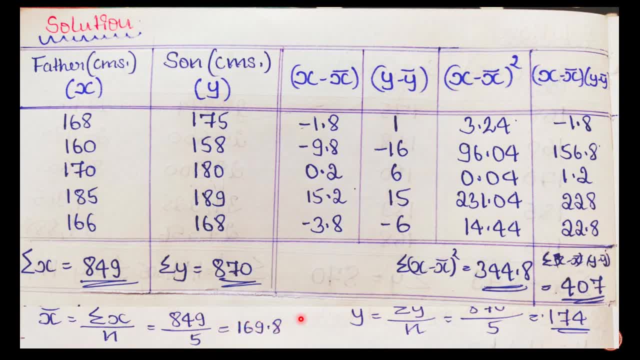 So x bar is equal to Sigma x, As in The total of x Divided by the number of observation in x, Which is: The total of x is 849 Divided by the number of observation 1,2,3,4,5, So which is 5. 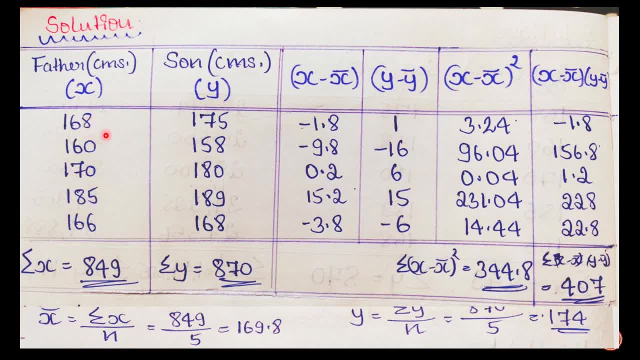 n is equal to 5. After doing this, We will get the value Which is the average value, Which is 169.8. Next now, Each of the x values, I mean This x bar value- We have to subtract from each of the x values. So in the first case, 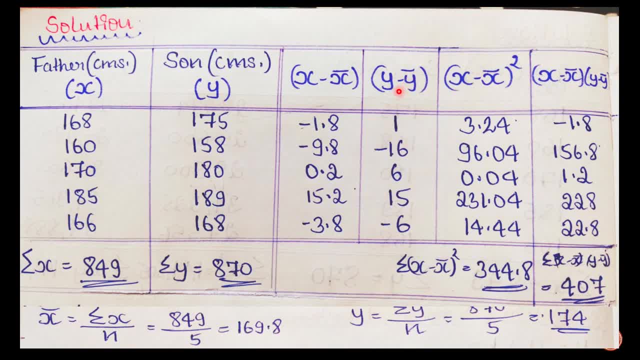 168 minus 169.8, So we get Minus 1.8. In the same way, You have to do it for every value, So you will get these values. After that, The next thing we need is y minus y bar. Okay, After giving y, Find out y bar. 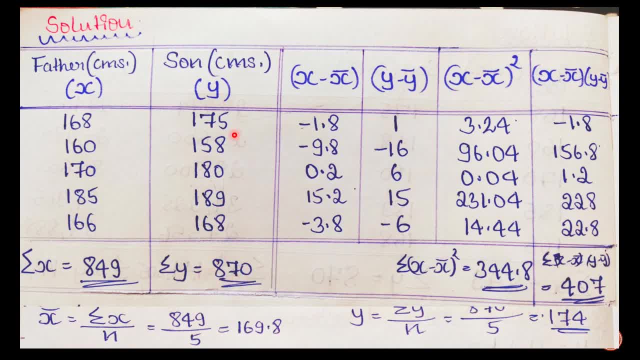 How did we find x? Find out x bar In the same way. y minus y bar- Okay, After giving y, Find out y bar. How did we find x? Find out x bar In the same way. y minus y bar- Okay, In the same way. Find out y bar for y. 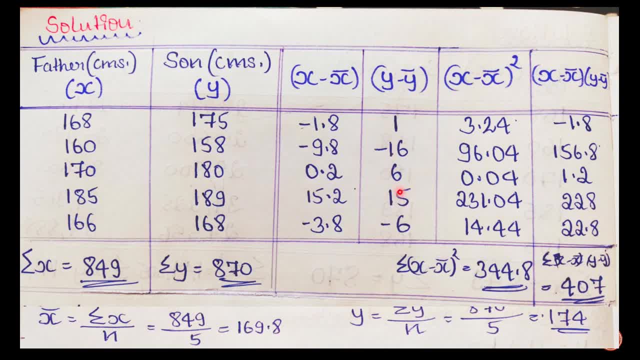 870 divided by 5, Which is equal to 174. After that, Each of the y values We have to subtract from this, So 175 minus 174, Which is equal to 1. In the same way, Find out each of the values. You will get these values. 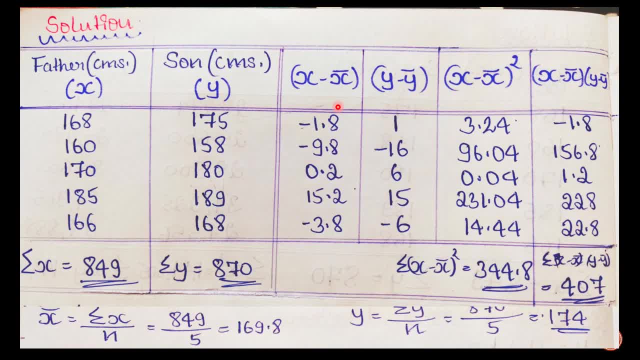 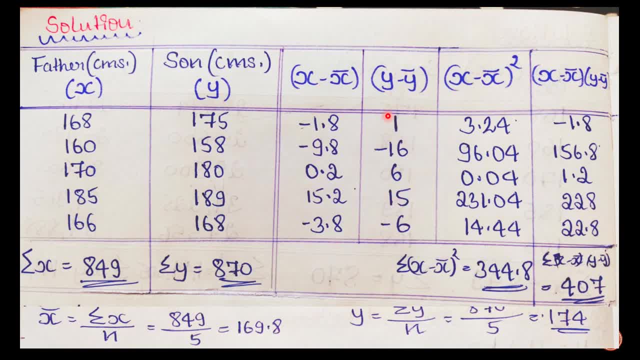 Square this Similarly For that Y minus y bar. The square is here Because We do not have A fitting equation As x on x, x on y. After that, We need a product for x minus x, x bar, Y minus y bar. Here, This Y minus y bar. multiply this. 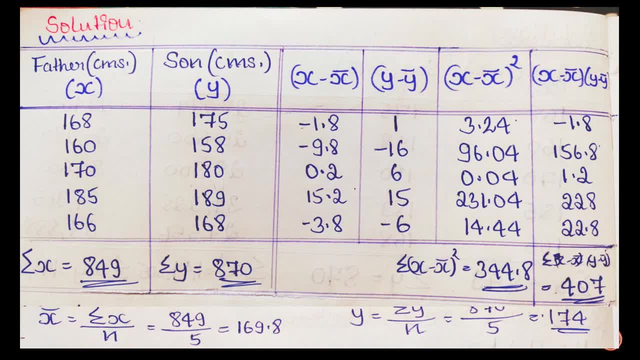 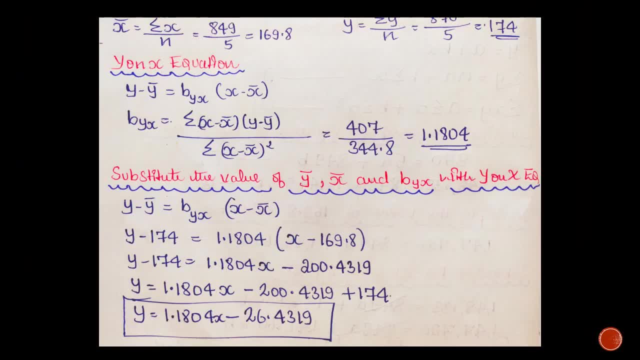 Got this. This wrapped up: x minus x bar into y minus y bar. That is 400 and 7.. So y on x equation is like this: y minus y bar. We have come up with this method, y minus y bar, which is equal to b of y, x into x. 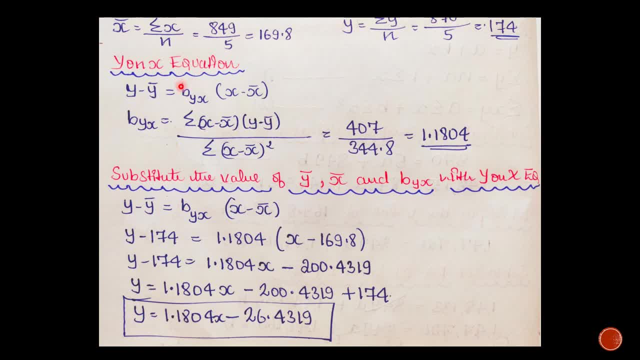 minus x bar. So first we need these values because we already know y bar. We have found out 174.. We also know x bar, 169.8.. The other value, or the only value which we need, is b of y x. 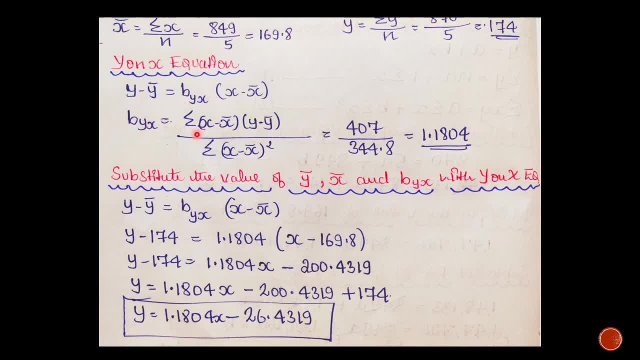 Directly. now we have to find out b of y x, which is sigma x minus x bar, into y minus y bar. We have found out which is equal to 407.. Then sigma x minus x bar square. So in the case of y on x, 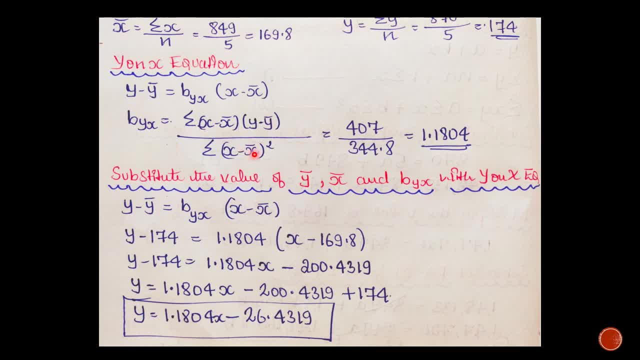 our denominator x is the value. Remember that 344.8 has come. Now, when we find out the quotient, we get a value which is 1.180.. This is our b of y x value. Even in the algebraic method we have the same value, So there will not be any difference in. 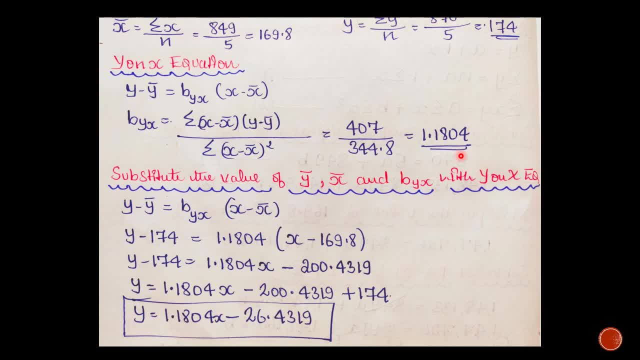 the values which you get when you apply algebraic method, and arithmetic mean method. There is no difference in the values After that. what we need to do is we have b value. What we will be doing is we are directly substituting that value with y on x. 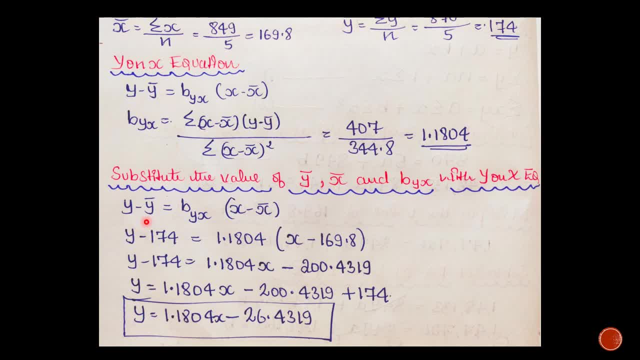 Equation. So we will be writing that y minus y bar is equal to b of y x into x minus x bar y bar 174.. We will multiply that y minus 174, which is equal to b of y x, is 1.1804.. 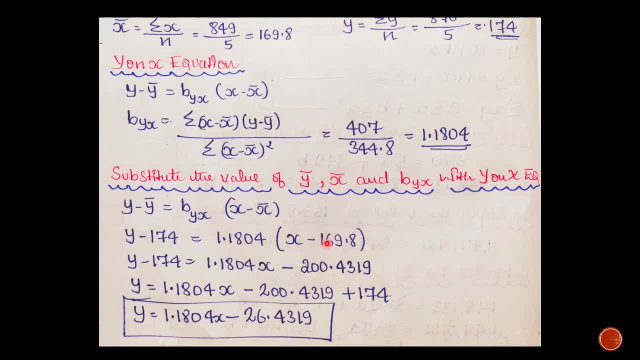 So we will multiply that, We will get x minus x bar, which is 169.8.. So we will multiply that Then next, what we will be doing is we will be multiplying this value with this part, x minus 169.8.. First we have to multiply 1.1804 by x. If we do that, we will get this value, 1.1804 x. 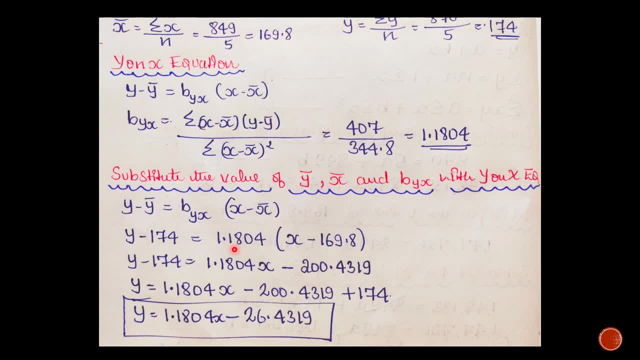 After that we have to multiply 1.1804 by minus 169.8.. We know that plus into minus is minus, So I will be writing that sign here. Then I will be multiplying 1.1804 with 169.8.. 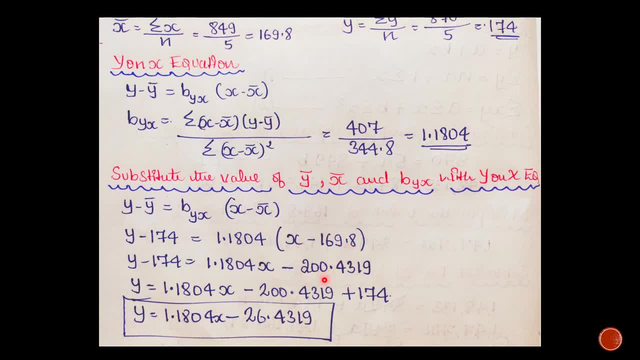 Which is equal to 200.4319.. After that I will put y here. I will put the numerical value here, So which will be: y is equal to 1.1804 x minus 200.4319.. Next, if there is minus here, if it goes to the right hand side, it will be plus. 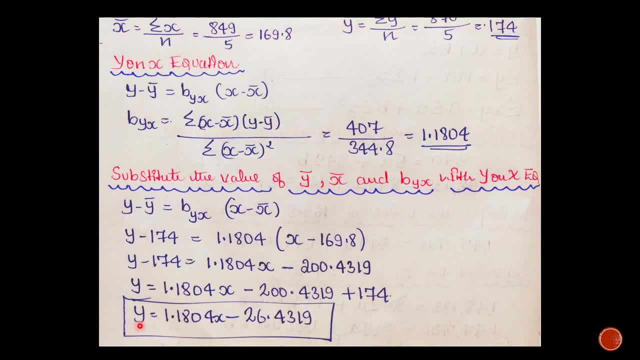 Plus 174.. Now we will get our y on x equation directly, Which is: y is equal to 1.1804 x minus 26.4319.. Here we can simply do the calculation in the arithmetic mean method. We can fit the y on x equation. 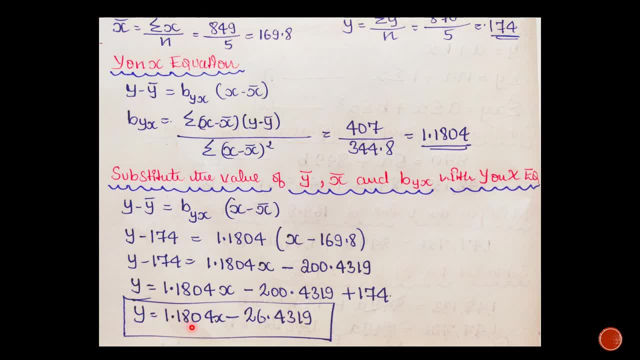 If you see, here 1.1804 is the b value and minus 26.4319 is the a value. So these are the values that come in the algebraic method. One difference is that first we get the a value there, After that we get the b value. Here we get the b value first and then the a value. 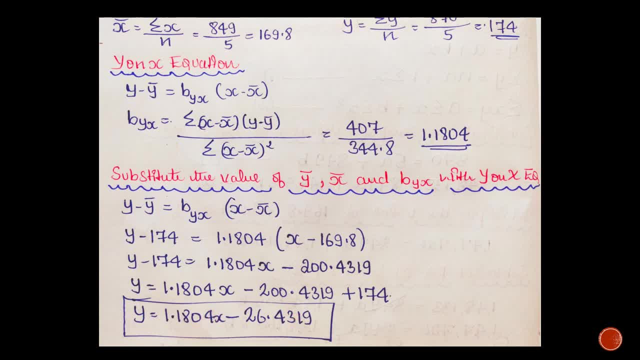 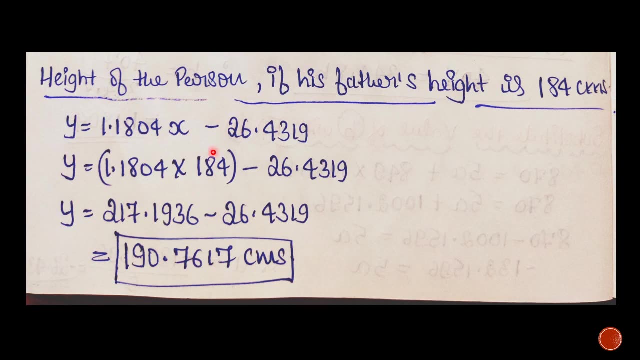 So this is the difference. Even with this equation, if you substitute the father's height, which is x value, then we will get the same result. So same Again. what I am doing is I have fit the y on x equation in the mean method, So I will be substituting x, value 184 with the y on x equation. 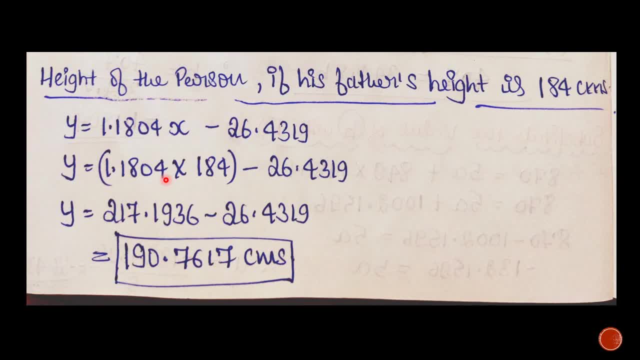 Arrive under arithmetic mean method, Our answer will be the same again: 190.7617.. Centimeter. So like this you have seen the computation in both the methods. So, like I said, the arithmetic mean method calculation becomes very easy. 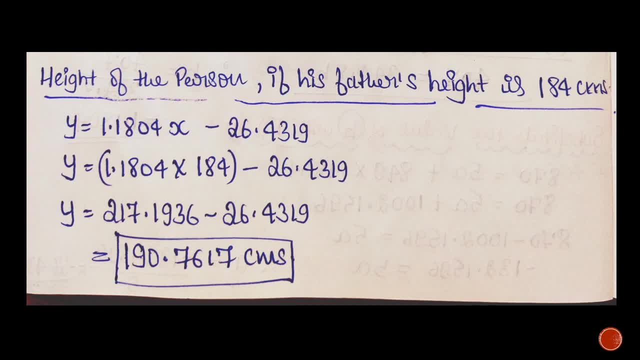 And at the same time it saves your time as well from examination point of view, Right. But what happened here is you get a value x, bar value, which had a fraction in it, Right? When fractional values come, it becomes difficult for us to do the computation. 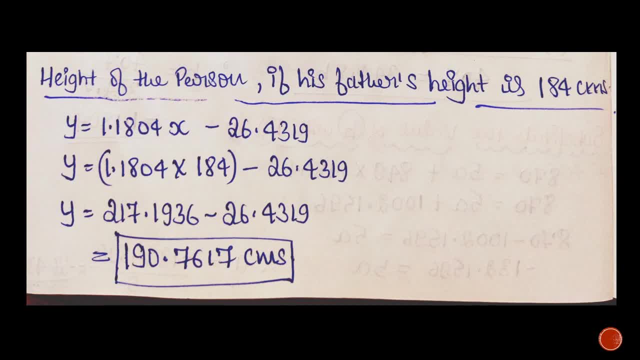 Even if you are using a calculator, You are using a calculator. Even if you are using a calculator, You are using a calculator. Even if you are using a calculator, You are using a calculator. But still, when you see a fractional number, you tend to forget some of the digits Right. 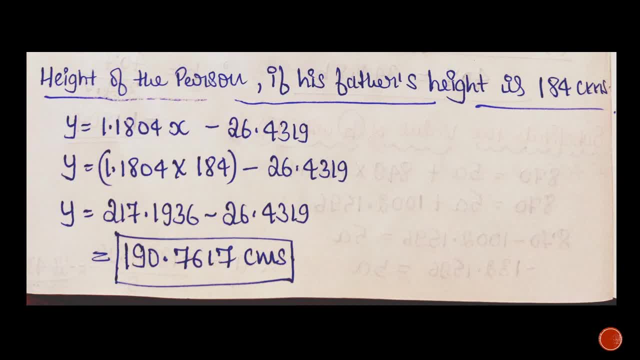 So if you do it like this, your calculation will become very difficult, But not difficult. So I urge you to use arithmetic mean method If the problem is silent about which method to apply. Generally people ask that kind of question. 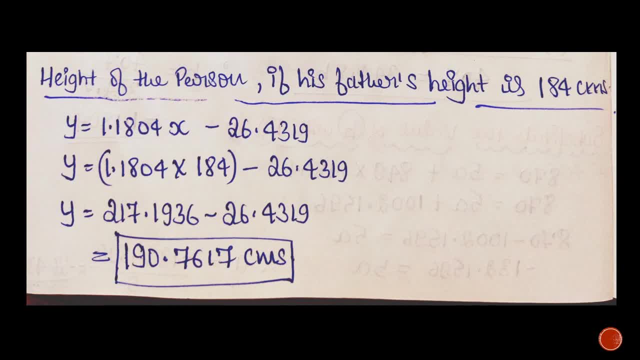 So the method is your choice. You are using the normal equation. I mean, if you are using the algebraic method to solve it, it is up to you, Or if you are using the mean method to solve it, it is up to you. 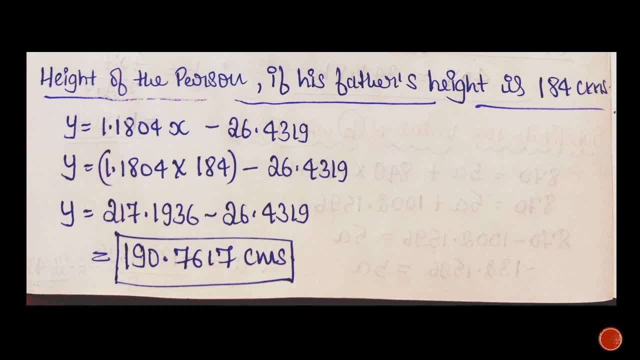 There. you don't have to ask in any way. You have to use this specific method to solve it. Okay, It is your choice. So I told you that when the x-bar fractional value comes, the computation becomes a little difficult from the mean method. 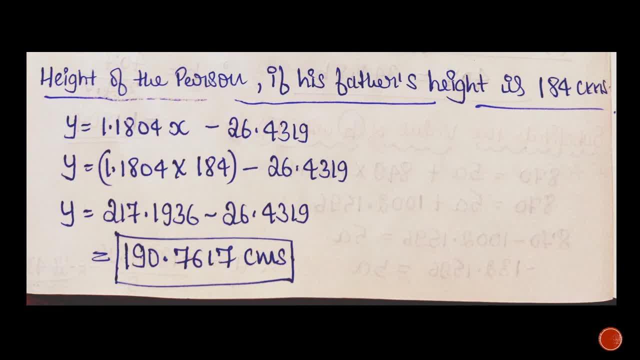 So instead, if you remember, when I discussed in my first video on regression equation the conceptual part There, I said: under arithmetic mean method, we use three kinds of equations to arrive at b's value, Which is Regression coefficient. 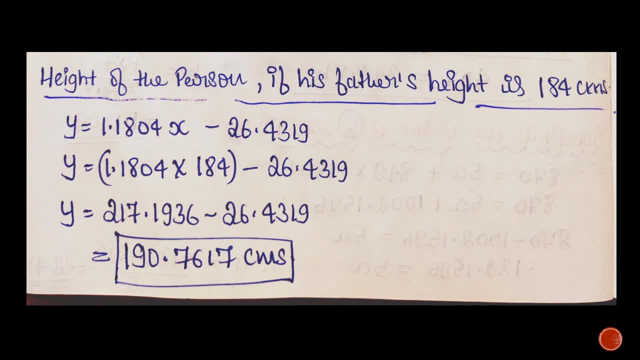 One, as we have done here, we have used x-bar value to find out that, And the other we use if information is given When they give correlation and standard deviation of x and standard deviation of y. That time also we can easily calculate b of yx or b of xy. 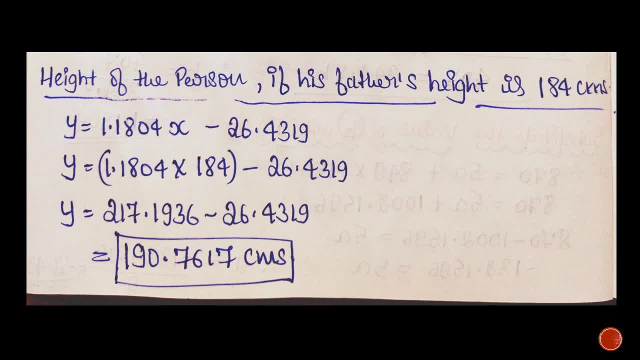 And another one. there was another equation, if you remember. There we are applying the direct method. Nothing but now x y, x, square y, square x, y, The way we find out the values in algebraic method. right. 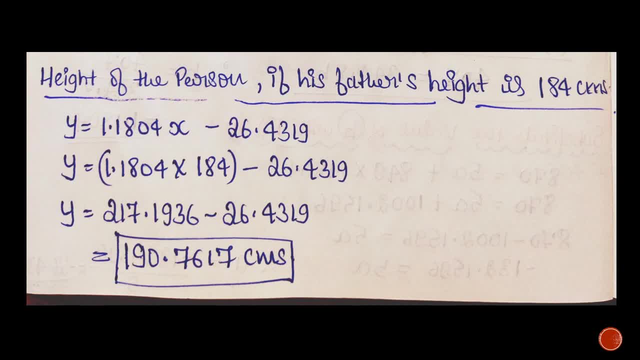 For the first time There is an equation that uses the same values. We can substitute for that. It is difficult for you to calculate x-bar value, So that is like this: At that time, the way we find out b of yx is: 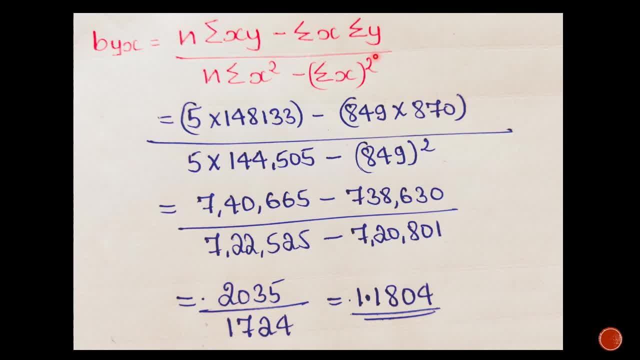 n is equal to sigma xy minus sigma x into sigma y divided by n, into sigma x square minus sigma x square. So come Your equation. When you look at the equation it is a little bit different Because there are many factors in it. 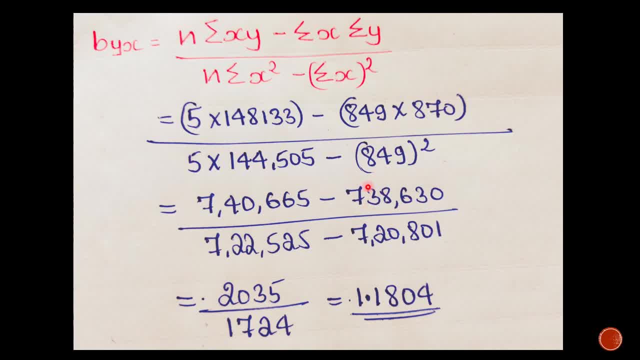 But again, the calculation will be easy. You can apply this too. Again, your b value will remain same. No changes will happen. Okay, So you can apply this equation as well, Or you can apply the previous equation with x-bar. 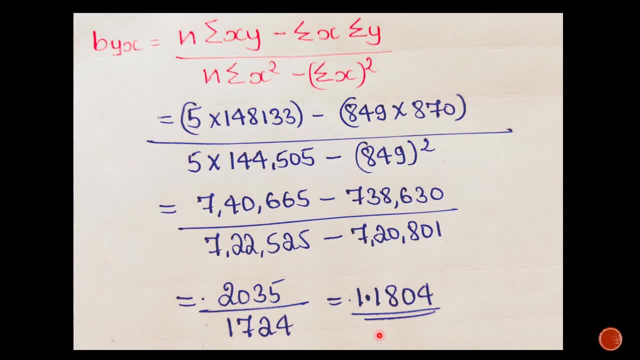 So you have to use that to do the calculation. After finding out this, even if you are applying direct method, That is, x y, x square y square xy, Even if you find out by using x y, The arithmetic mean method is that we need x-bar and y-bar values. 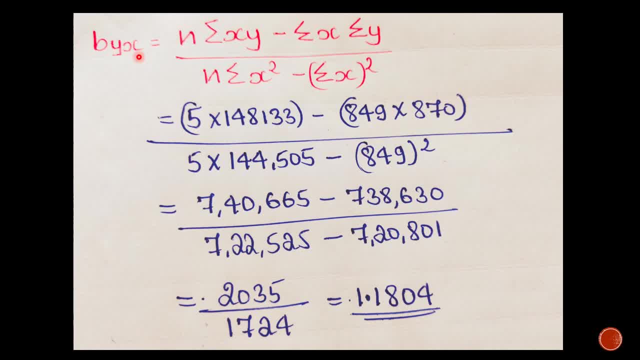 Because when we consider the y on x equation, y minus y-bar, which is equal to b of yx into x minus x-bar. So if the value of x-bar and y-bar comes there, You have to compute that additionally If you are going with this direct method.